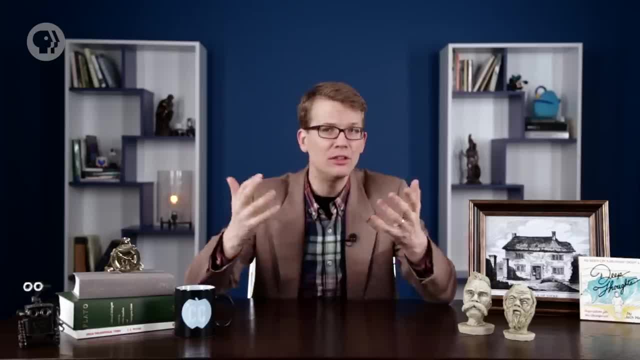 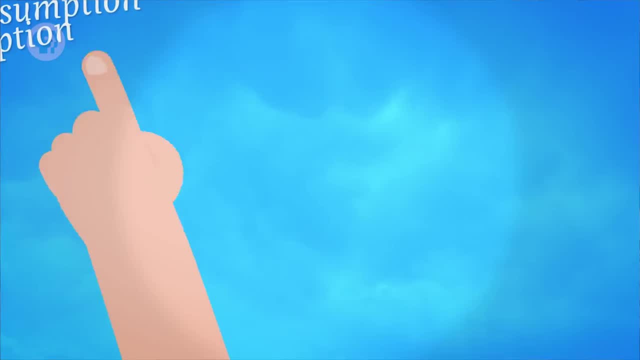 accountable for them. Yeah, it's going to be that kind of journey. Rather than just looking at the world and describing what we see, we'll be evaluating it. We will take nothing as given, set our assumptions aside, or at least try really hard to and do our best to see the world. 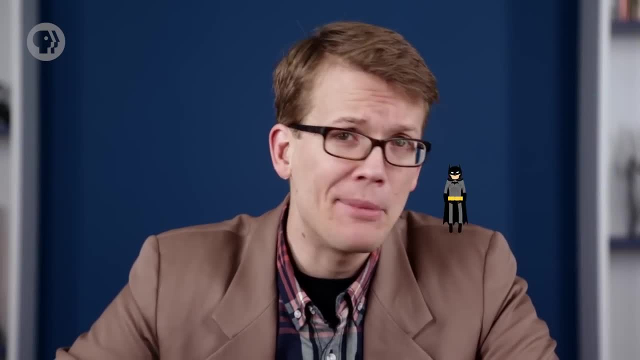 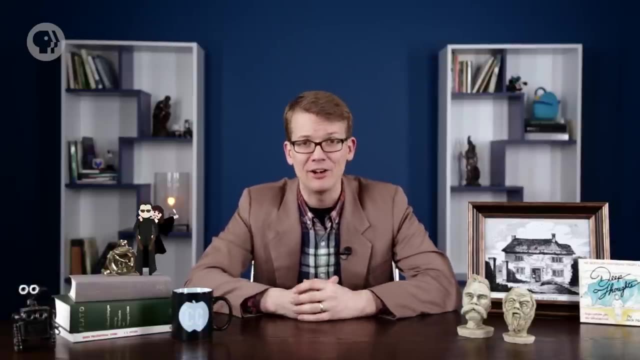 as if we've never seen it before, And for what it's worth. we'll also be talking about Batman and what Dick Grayson can teach us about the concept of identity, And we'll learn how the Matrix can help us understand the life and writing of Rene Descartes. Also, we'll try to answer unanswerable. 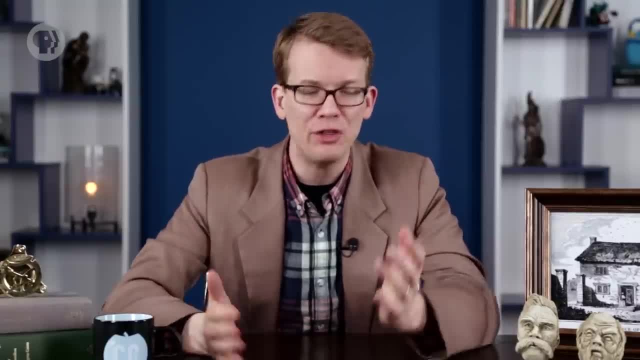 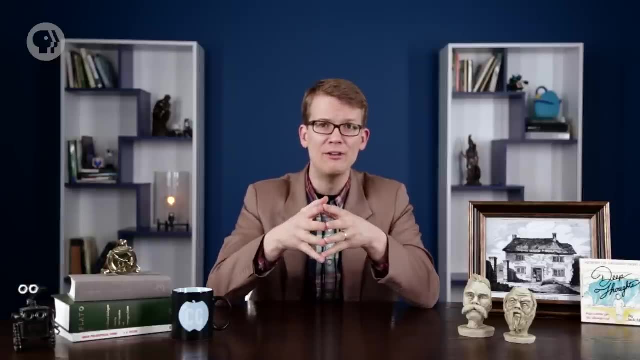 questions and puzzle over paradoxes that have plagued geniuses for thousands of years. It's going to be hard and enlightening and frustrating, and if I do my job properly, it'll stick with you long after you and I have parted ways Because we are going. 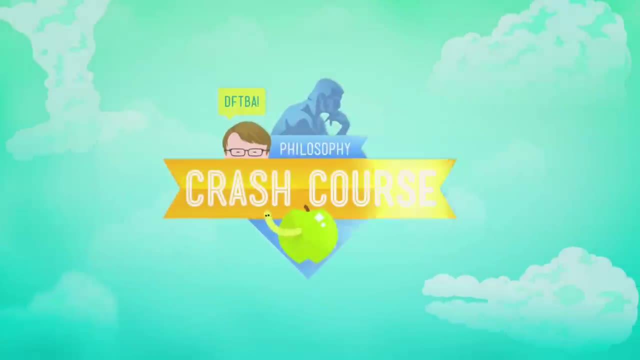 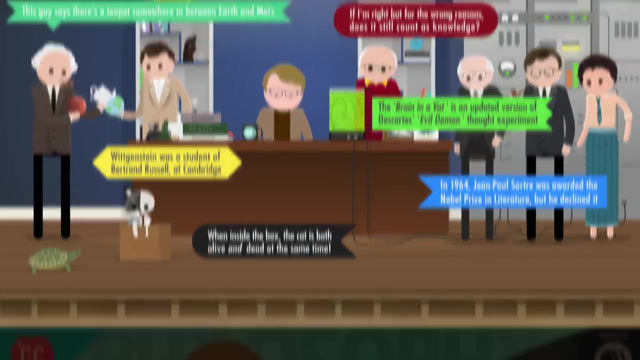 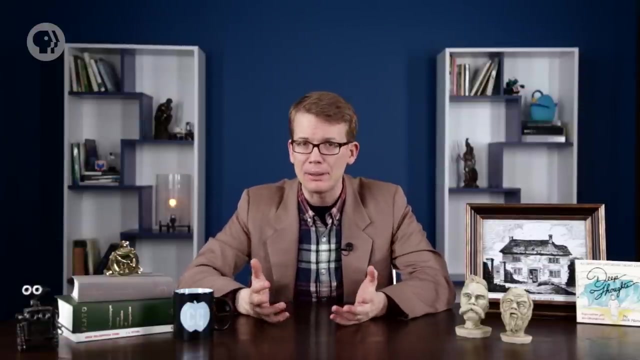 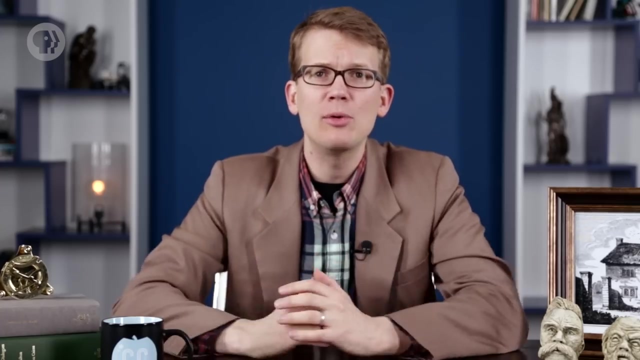 to do philosophy. These days, people use the word philosophy to describe some opinion they might have or an approach they have to a certain topic. Like you might have a philosophy when it comes to golf, though I personally do not- But we are going to use this word more narrowly to describe a way of approaching the world. 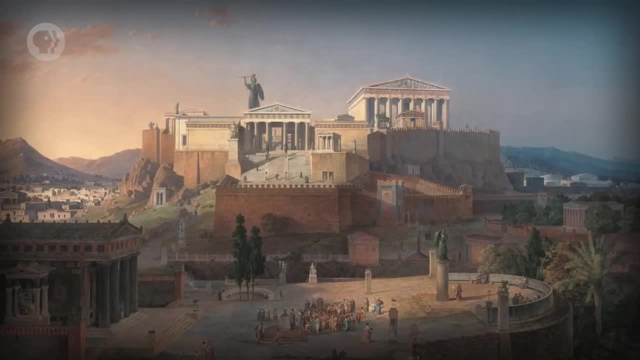 that traces its roots back to ancient Greece, 500 years before the Common Era. This was a time of great intellectual movement around the world. Buddhism and Jainism were developing in Asia at the same time. Philosophically, it was a time of great intellectual movement. Buddhism and Jainism were developing in Asia at the same time. Philosophically, it was a time of great intellectual movement around the world. Buddhism and Jainism were developing in Asia at the same time. Philosophically, it was a time of great intellectual movement. 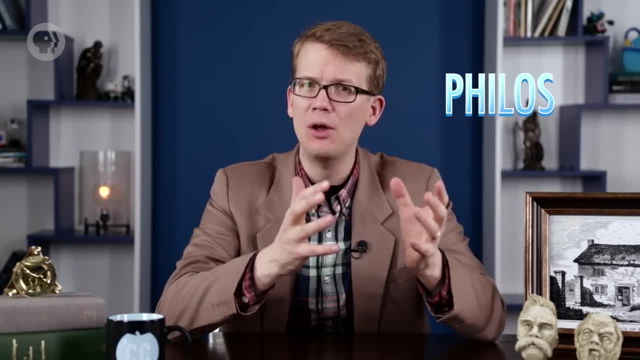 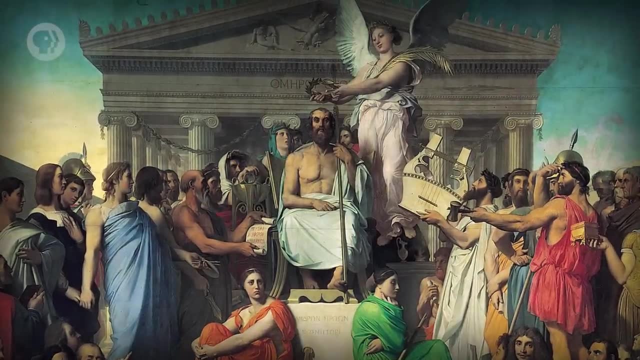 There, scholars were tangled up in a distinction they were just beginning to make between philos and mythos, or what we'd now roughly call science and storytelling. At that time, there were bards like Homer who were trying to understand and explain the world through 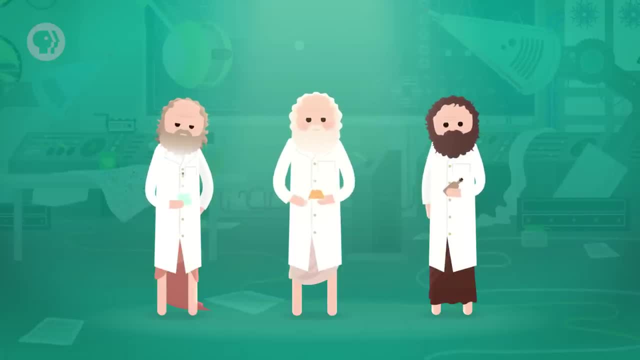 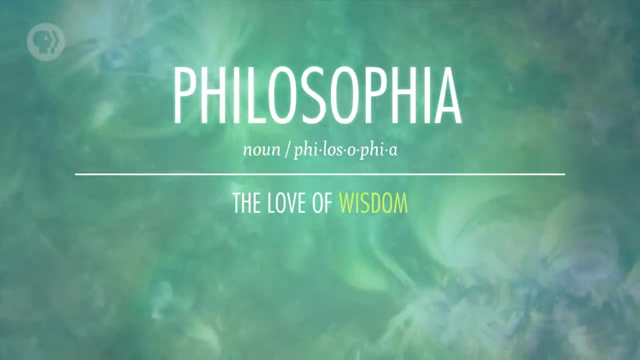 stories, while the earliest philosophers were using methods that were more analytical and scientific, although they didn't really have the concept of science back then. So philosophia, literally the love of wisdom, was a new way of trying to make sense of the 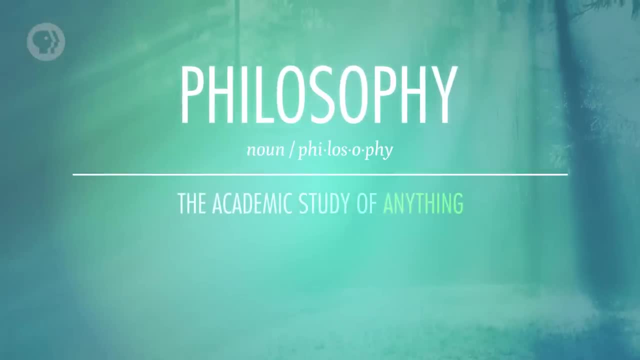 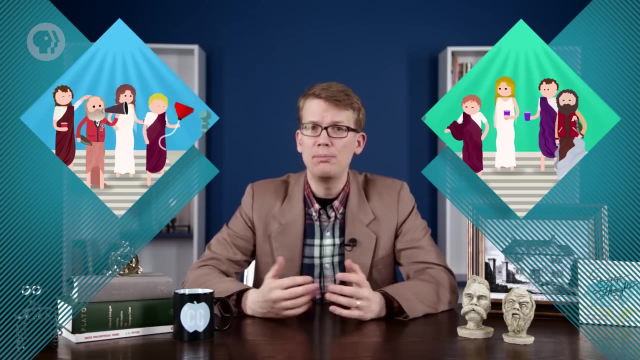 world. When the earliest philosophers used the word philosophy, they basically meant the academic study of anything, Which, like I guess, could include golf, But at what we might call the first universities in the Western world: Plato's Academy and its rival Aristotle's Lyceum: math, biology, physics, poetry, political science and astronomy. 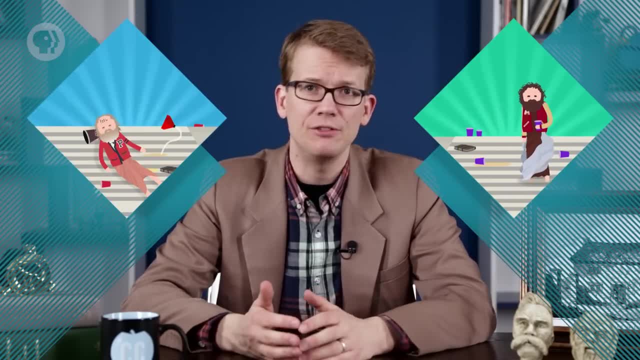 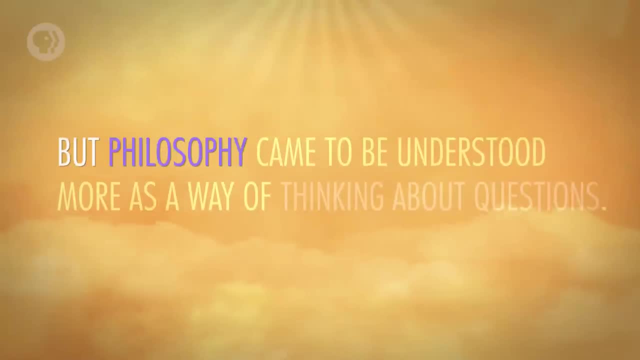 were all considered to be philosophy. Eventually, scholars began thinking of these fields differently, as separate disciplines. Studies that had strong empirical elements came to be considered science, a search for answers, But philosophy came to be understood more as a way of thinking about questions, Big questions. 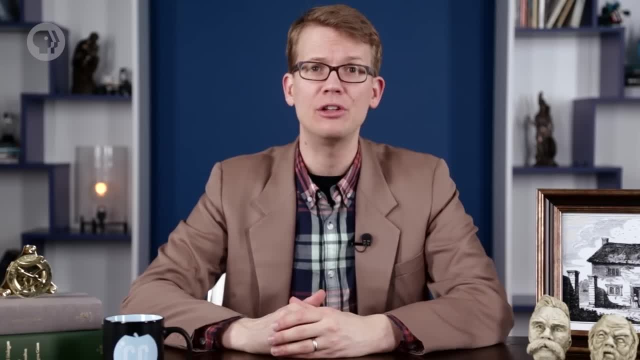 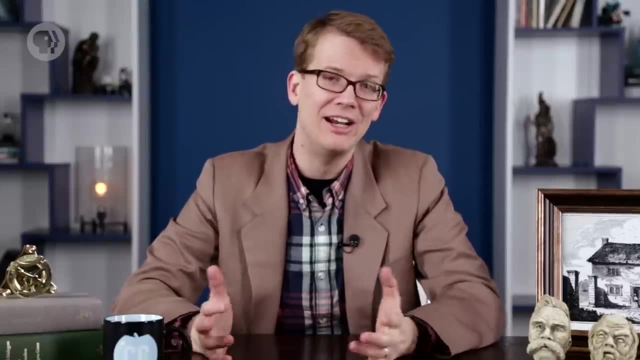 Big questions And today, 2,500 years after the ancient Greeks first brought them up, philosophers still love asking questions, oftentimes the same questions, and they don't mind that they never get an answer. So what are these big questions that have managed to intrigue and stump philosophers? 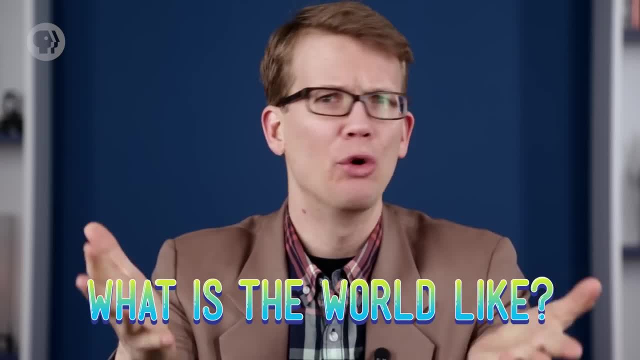 for so long. One of the first might best be phrased as: what is the world like? Sounds simple enough to answer, right Like just look around and see all the stuff. Well, this is what the world is like. 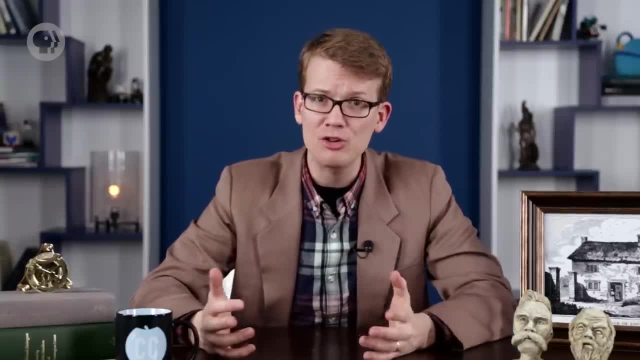 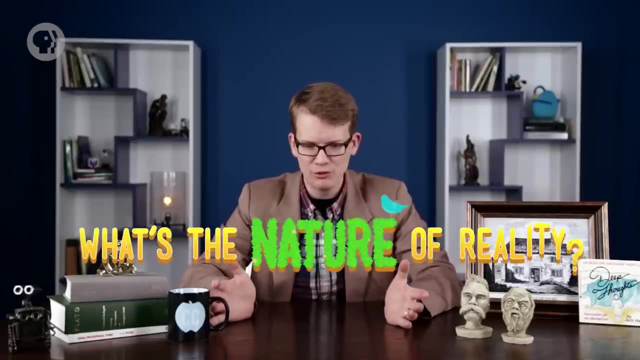 But the philosophical approach isn't just based on observation. It has other, much more complex questions packed into it. When a philosopher wonders what the world is like, she might really be asking: what's the nature of reality Like? is the world just made up of matter and energy, or is there something else going? 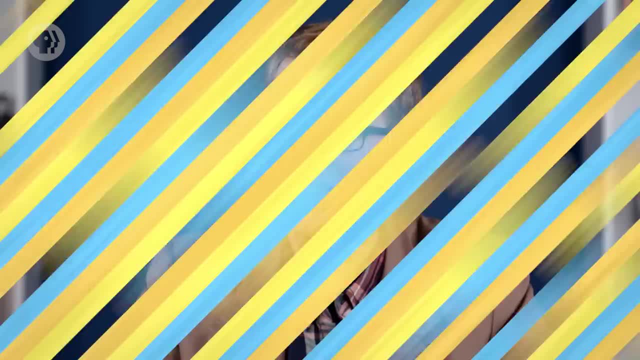 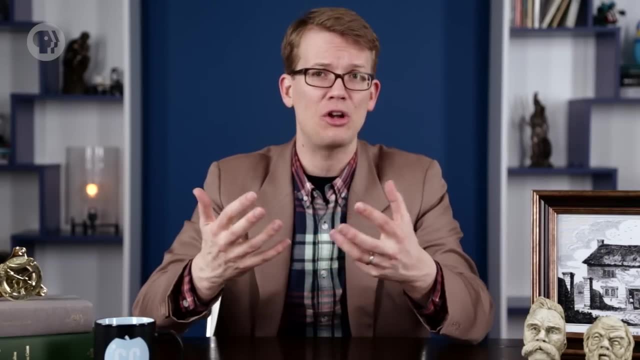 on. And if it is just matter and energy, then where did it all come from? Is there a god? And if so, then what is he or she or it like? And, for that matter, when you're asking about the world, can you also be asking about the nature of yourself as a citizen of the world? 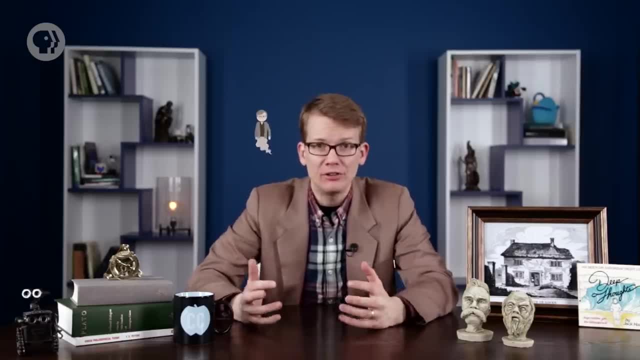 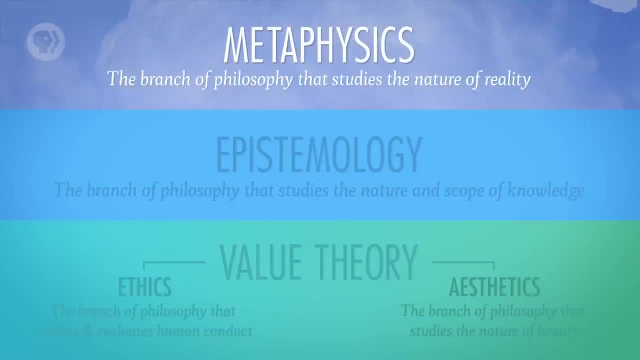 So what kind of being am I? Do I have a soul? Is there something immaterial about me that survive after I die? All of these questions are ways of exploring what philosophers call metaphysics, one of the three main branches of philosophy, an effort to understand the 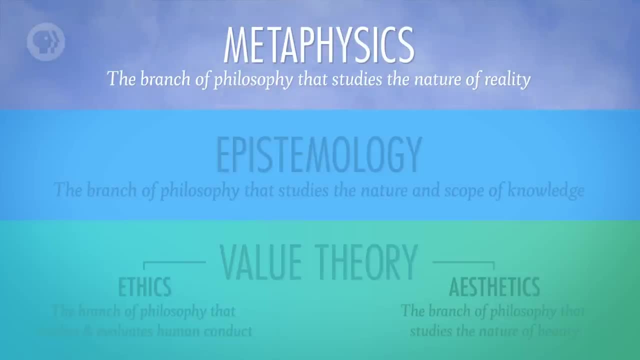 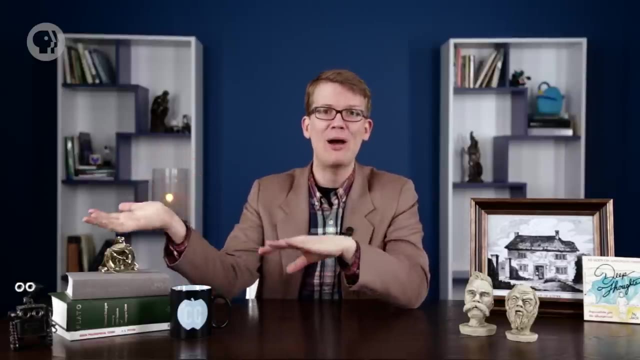 fundamental nature of the world, of the universe and of being Now. if those questions aren't heady enough for you, we, as students of philosophy, also have a whole separate set of questions that are about how we know the answers to any of. 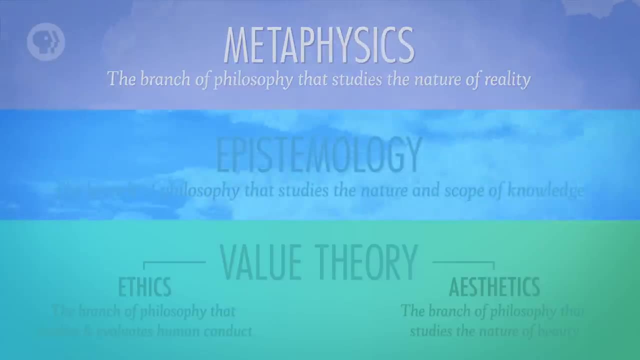 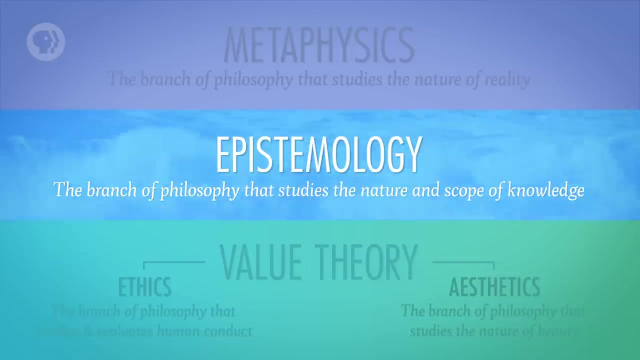 this stuff, This particular strain of philosophy, which is like knowing about knowing, is epistemology, literally the study of knowledge, the second major field of philosophy, And it poses questions like: is the world really what I think it is Like really is? 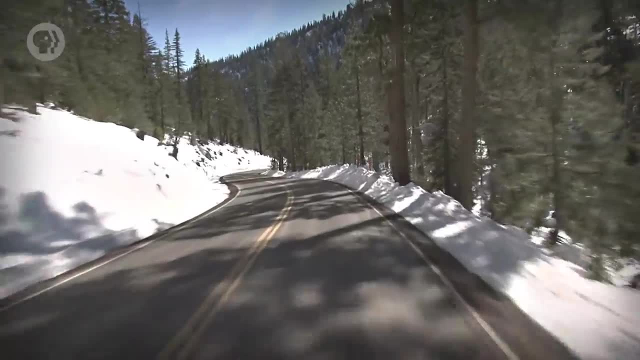 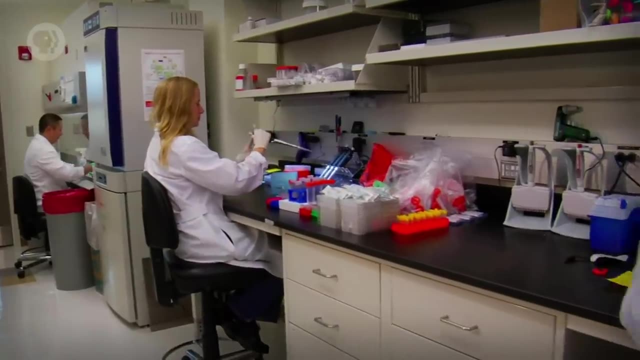 everything I see and think and experience is it actually true? If it isn't, then what is true, and what's the best way to go about figuring out the truth? Is science the best way, or are there more ethereal paths to truth, paths that science can never really travel? 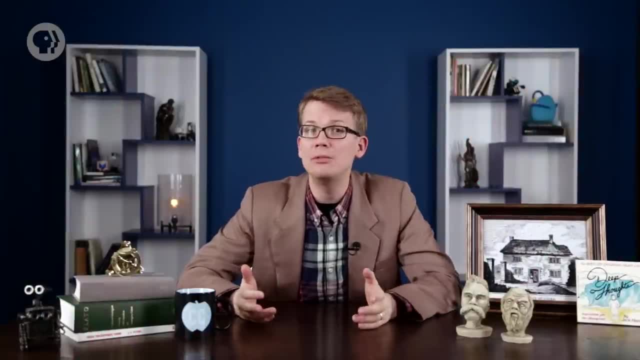 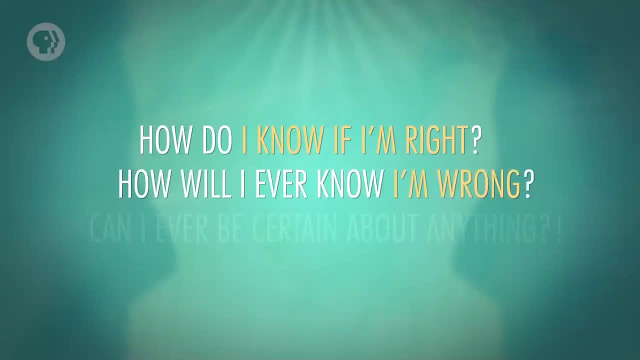 And let's say that after a lot of searching and question-asking, I begin to develop some ideas, like an inkling about what might be true. Then how do I, How do I know if I'm right? How will I ever know I'm wrong? 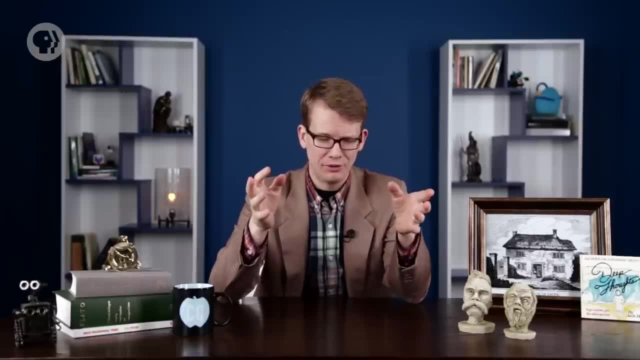 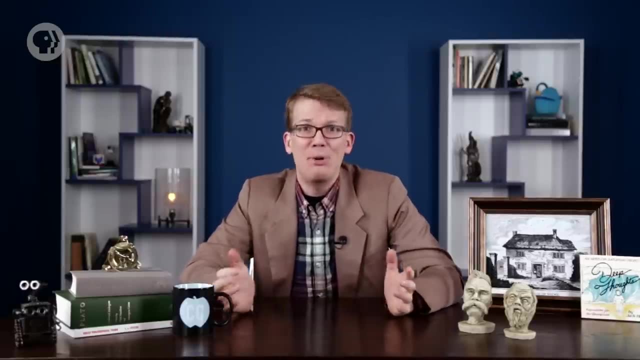 Can I ever be certain about anything? Now, at this point I wouldn't blame you if you're thinking: am I real, Do I, do I know anything? Well, as questions go, these might not seem super practical, But there's another area of philosophy that helps frame your thinking around what you. 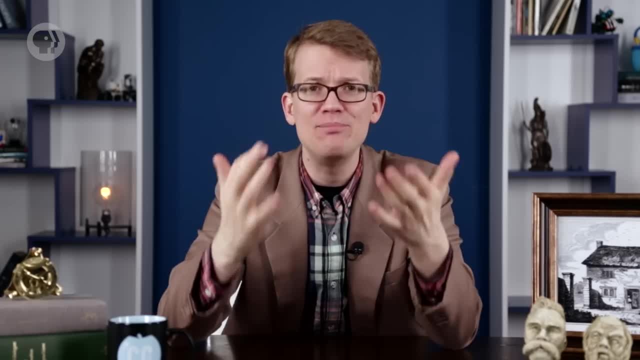 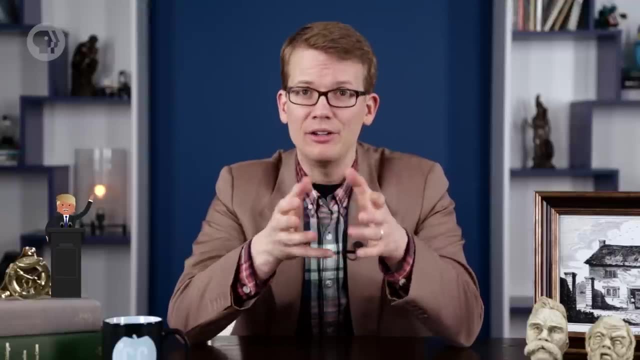 actually do, Like how you should act and what you should attach meaning to. It's called value theory, and it's usually divided into two main branches. The first is ethics. You've heard of it. it's the thing that politicians are always. 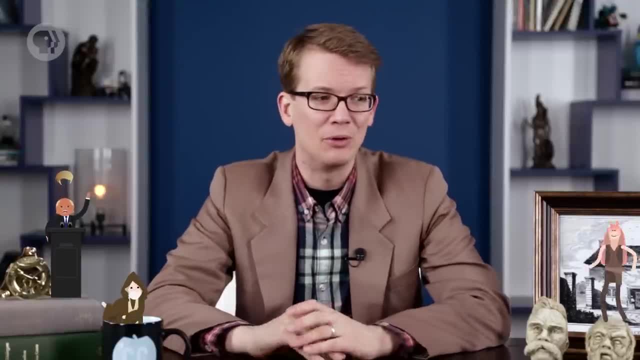 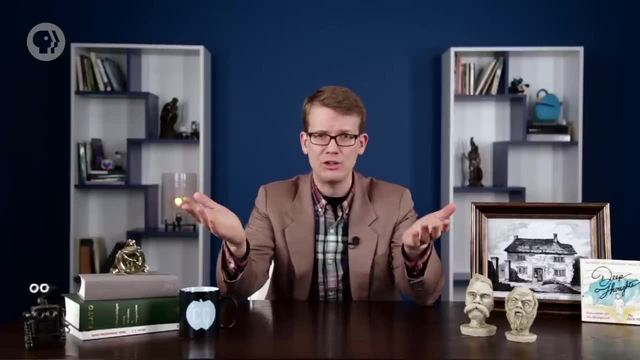 said to lack, and Jedi are supposed to have in great supply. Though don't get me started on the prequels. In philosophy, though, ethics isn't just a code of what's right and what's wrong. It's the study of how humans should live with each other. 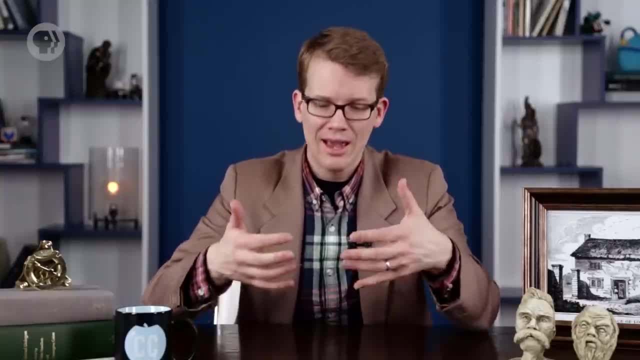 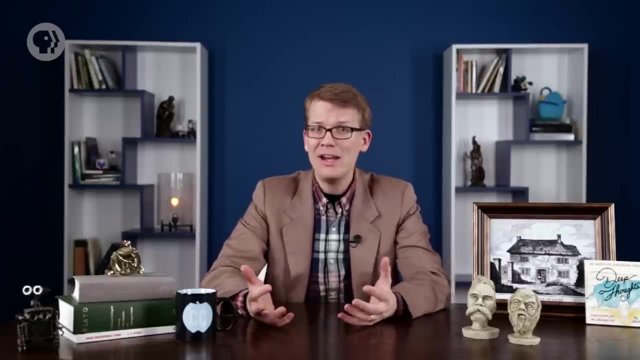 Rather than just sitting around and judging people. ethics involves posing questions like: how should I live? Is there any reason that I should treat, say, strangers differently than the people I love? And, for that matter, do I owe anything to myself? What about animals? or the Earth? 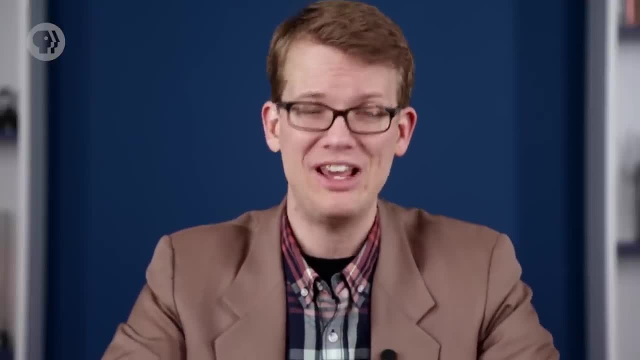 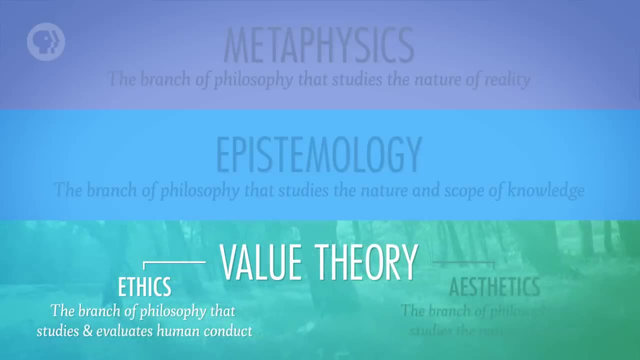 And if I do have any of these obligations at all, where do they come from? Who says Ultimately, whatever system you use to decide what's good or evil, as human behavior goes, is determined by your values. That's why ethics is considered part of value theory. 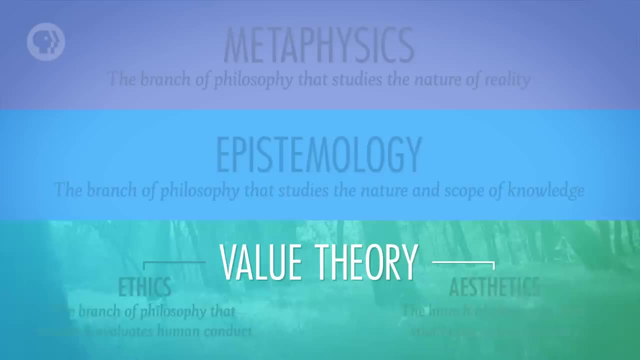 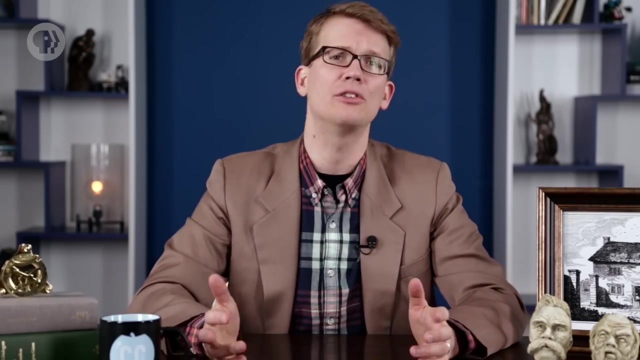 But the other part of value theory isn't about what's right. It's about what's beautiful. Aesthetics is the study of beauty and art. Now, the concept of beauty is talked about practically everywhere, from the media to art school to barber college. 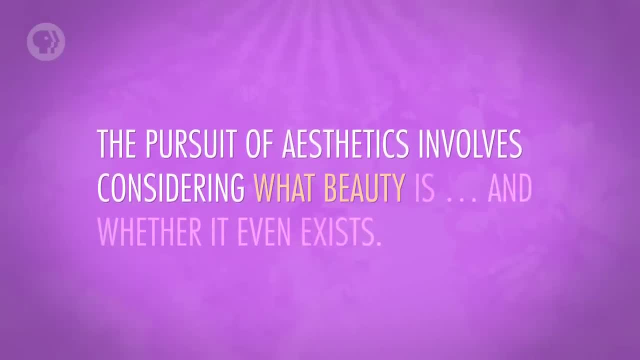 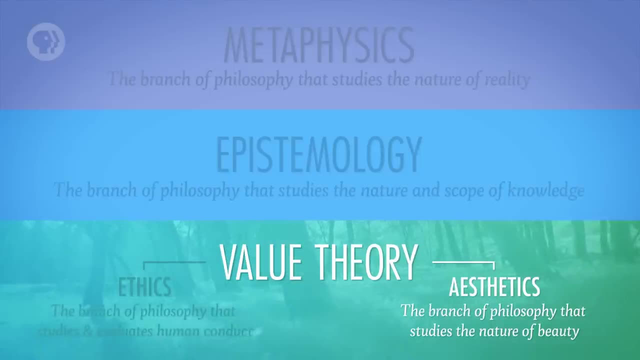 But for philosophers, the pursuit of aesthetics involves considering what beauty is and whether it even exists. Aesthetics is a part of value theory, because beauty and art are the same thing. It's the same thing. They're things we value and evaluate. 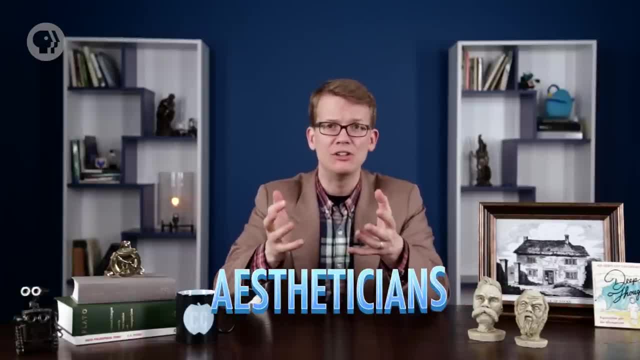 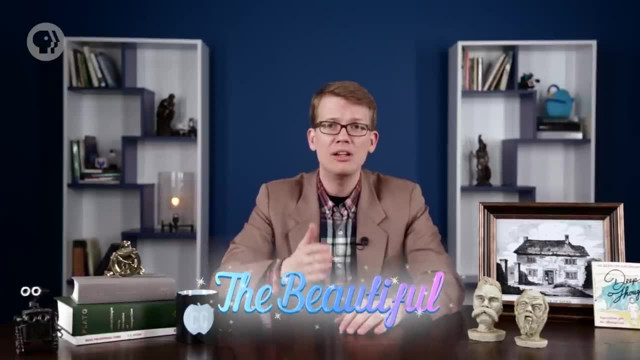 And many people who study this particular kind of philosophy, known as aestheticians, believe there is such a thing as the beautiful, Something that doesn't just depend on what you happen to find attractive, but something that's just objectively true. And finally, there's one more aspect of philosophy that I should mention, because it doesn't. 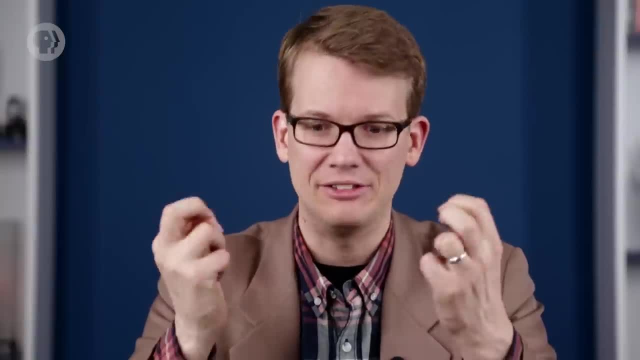 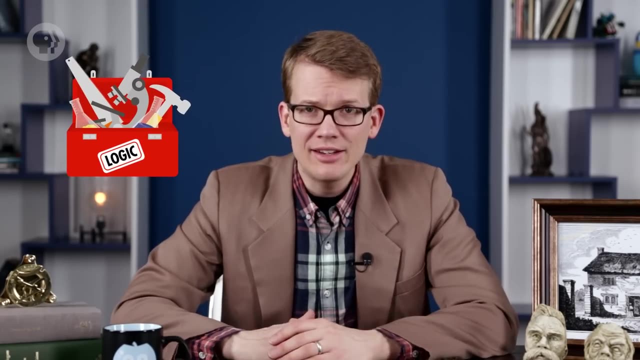 ask questions so much as help us find answers. Yes, finally some answers. And that thing, which I happen to think can be beautiful in its own way, is logic. Logic is the philosopher's toolbox. It contains the saws and hammers, the microscopes and beakers that philosophers use to go about. 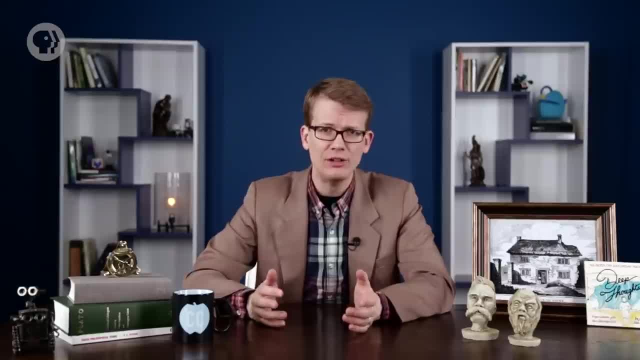 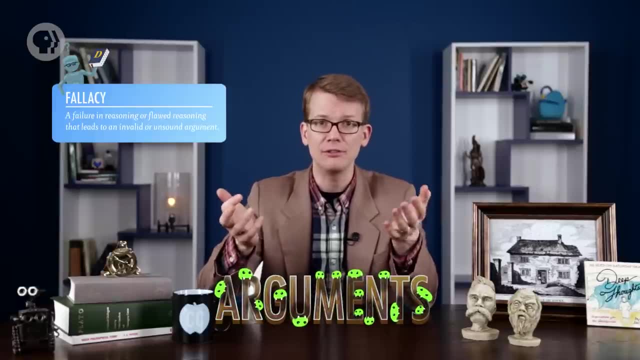 answering their questions in a clear, systematic way. Logic is about reasoning, giving strong arguments that don't fall victim to fallacies which are, as you will learn, the mortal enemies of philosophical precision. Okay so, metaphysics, epistemology, value theory, they might all seem pretty airy and 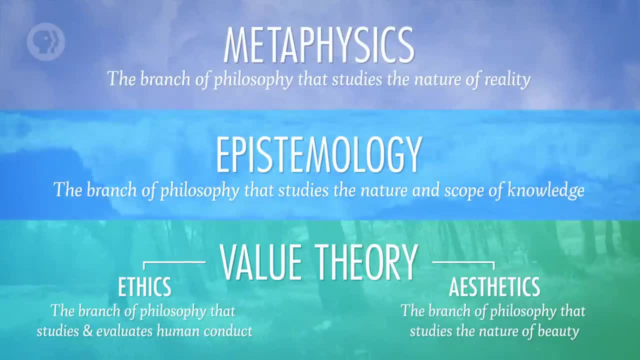 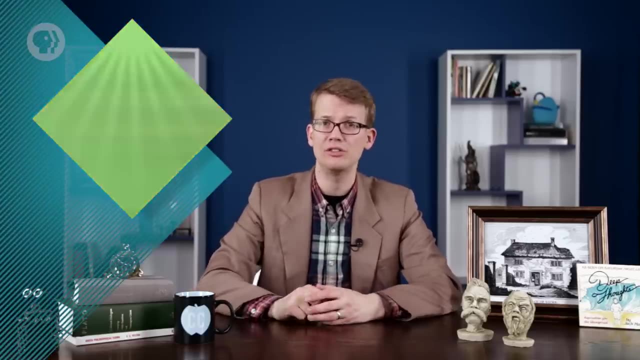 abstract. But don't worry, because you have already done philosophy. even though you might not realize it, You do it in almost every aspect of your life. Every time you argue, you argue. Every time you argue with your parents or wonder if you should date someone or decide. 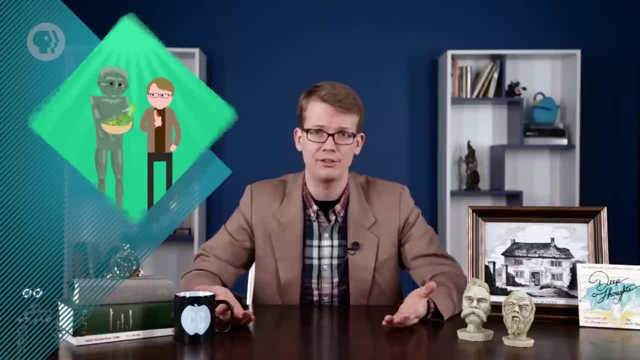 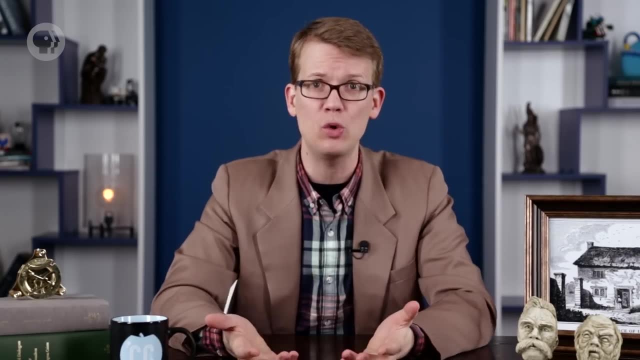 to eat a salad instead of a ham and cheese hot pocket. you are doing philosophy Because you're thinking about the world and your place in it. You're figuring out what you value, why you value it and what you should do about it. 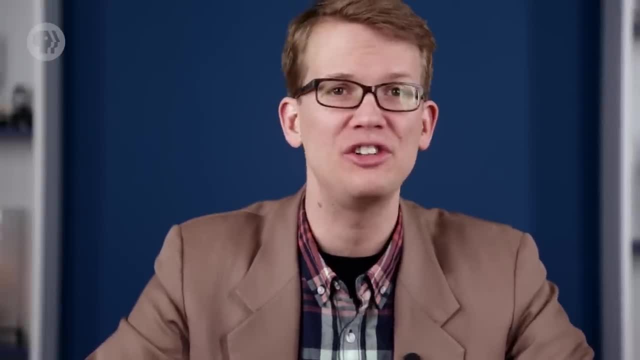 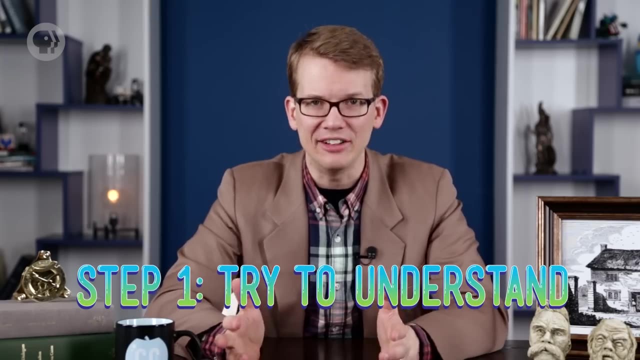 So here's our plan. We're gonna learn about the major fields of philosophy, posing questions and considering possible answers along the way, and each time we will use a two-step method. First, we'll really try to understand. You're not gonna agree with all of the ideas that I present to you. 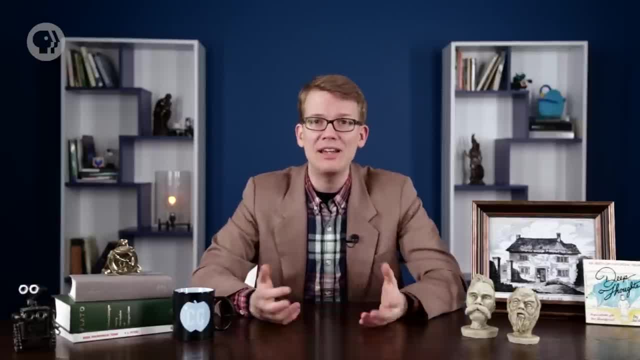 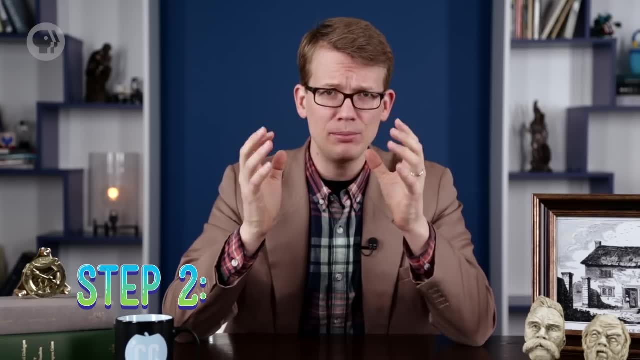 And I won't agree with them either. That's not the point. The point in step one is to really try to get inside of an idea, to understand it as charitably as possible. Then in step two, you'll subject your understanding to some serious critical evaluation. 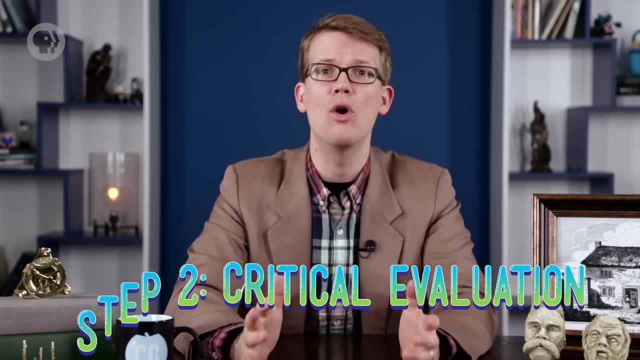 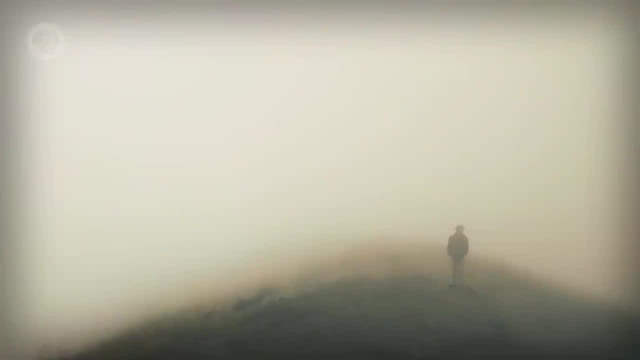 Basically, you'll try to knock down what you think you know about a particular view of the world, And you'll do this whether you agree with the view or not. Why? Because only when you challenge your understanding of how some people view the world can you. 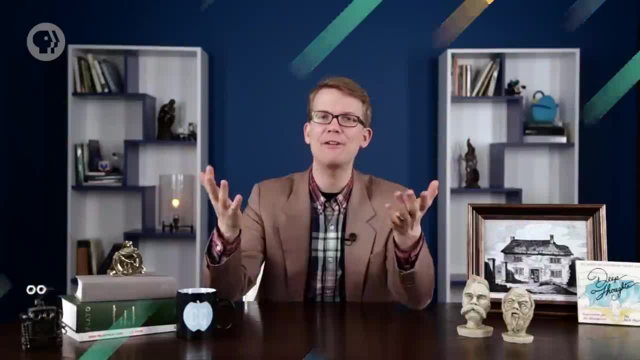 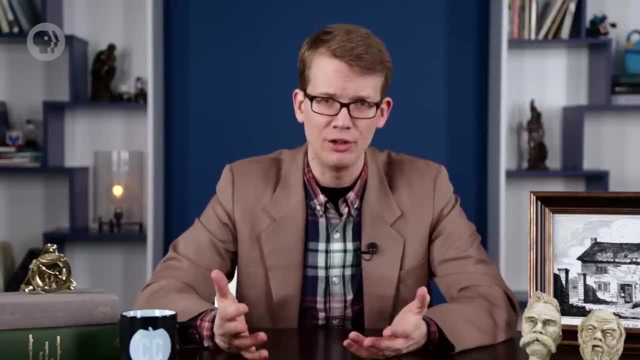 decide for yourself if theirs is a view worth having. Which leads me to my final point. Philosophy is not your usual field of study. I'm not gonna be teaching you a body of knowledge where success means you know a bunch of stuff. Success in this course will mean that you know how to think.